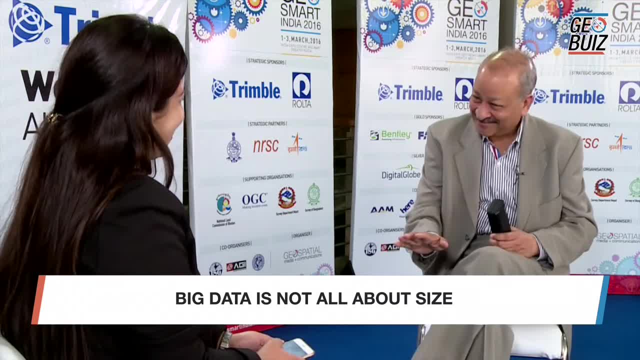 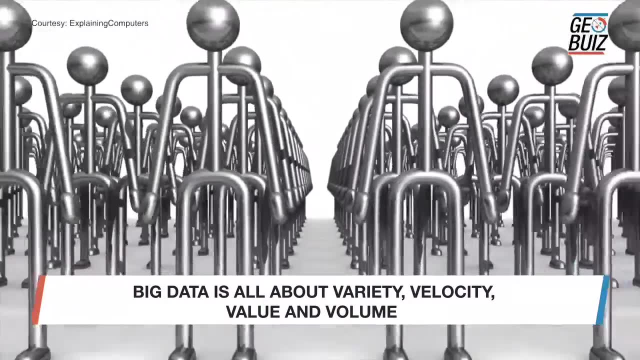 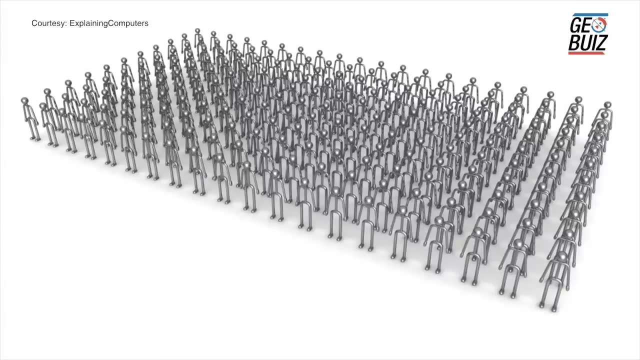 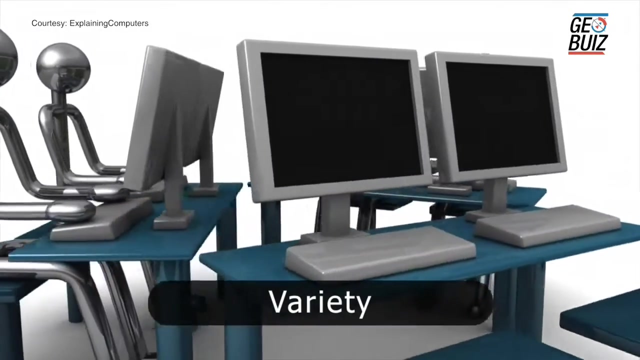 has something to do with size, So it's not necessary. So big data is all about the variety and the velocity of the data that we have today, Not the volume, Not the volume alone, Volume, of course. So volume, velocity and your variety Today, volumes. 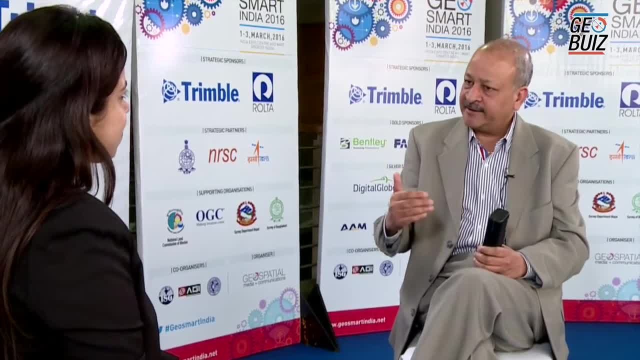 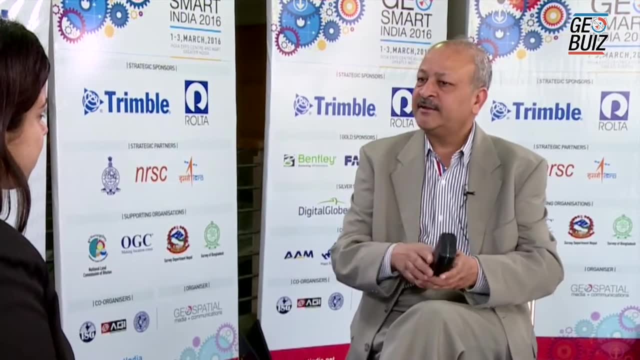 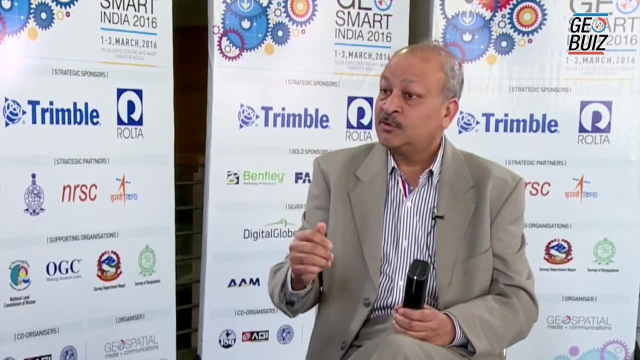 have been all throughout. But in today's context you have very different kind of data which is available, Like there used to be structured data, Then there used to be unstructured data, Now you have data like your media, your audio video, your social, your sensors And 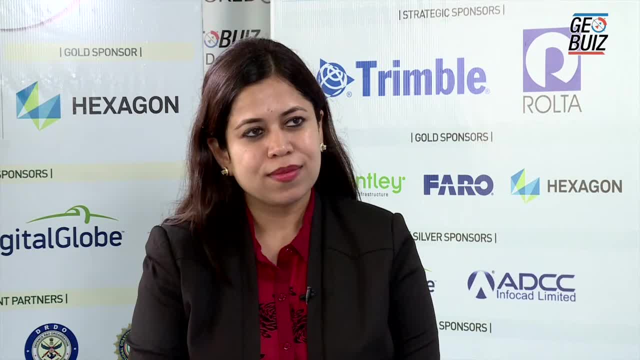 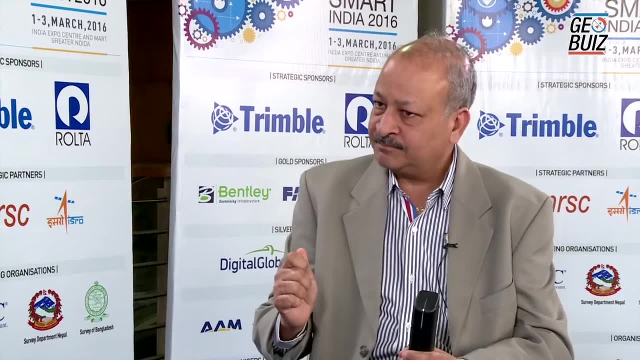 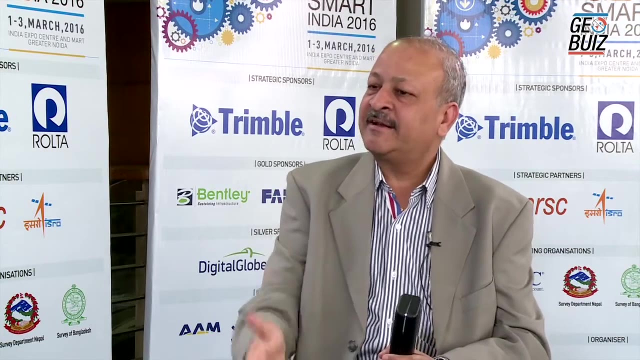 when I say velocity today, some of the places, when you look at cameras or you look at sensors, you see the volume and the speed of the data It, you know, transmits. That is what you need to deal with. So when we say big data, it is actually called traditionally three. 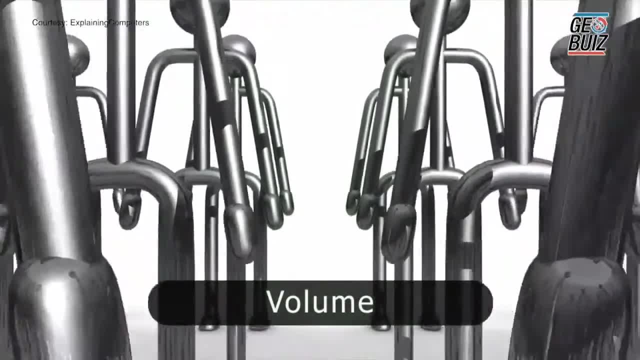 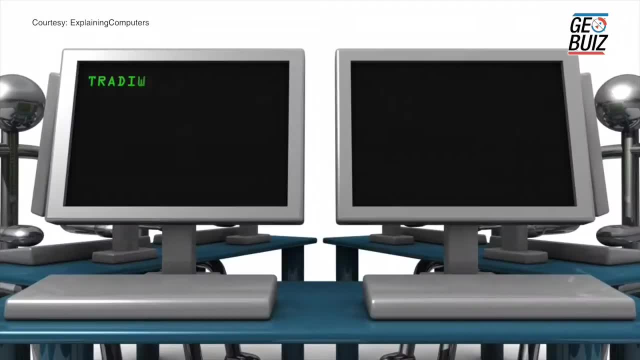 Vs, and now the fourth V has been added. So we say volume, velocity, variety, and now we have said the fourth one, the value. What is the value we derive out of all these? That is all about big data, to start with. So how do you see it as? 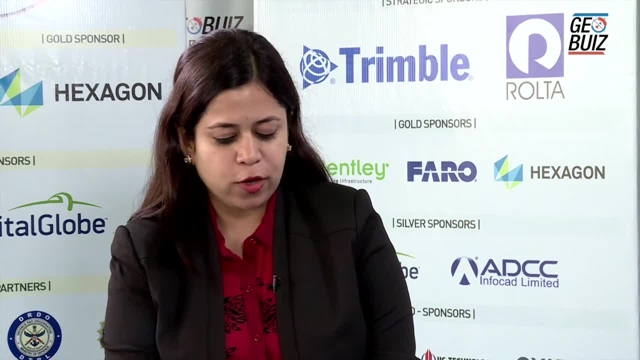 In its report on big data, McKinsey Global has said that it is the only big data. The highest value is the data that is gathered in the digital media And theuest one. the Global Institute estimates that location data level stood at 1 petabyte in 2009 and had 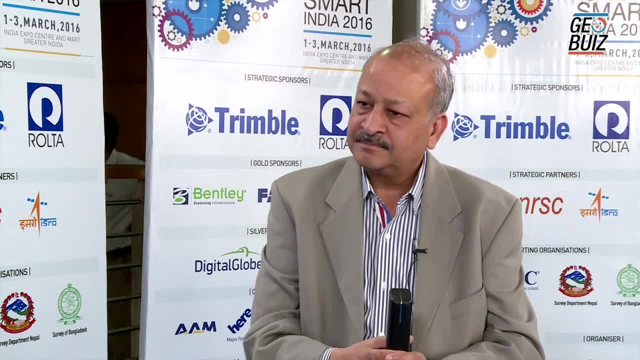 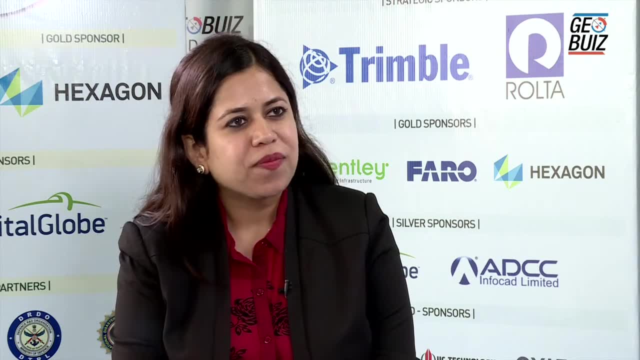 a growth rate of 20% per year. This did not include data from RFID sensors. It also does not include dark data. So what is the amount of data we are really looking at? So if you ask me really, your imagination will be the data science, And that's where 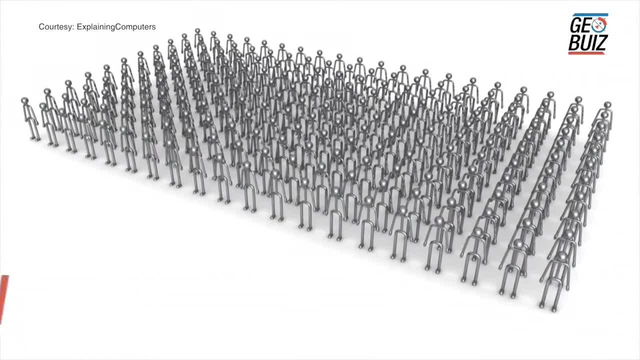 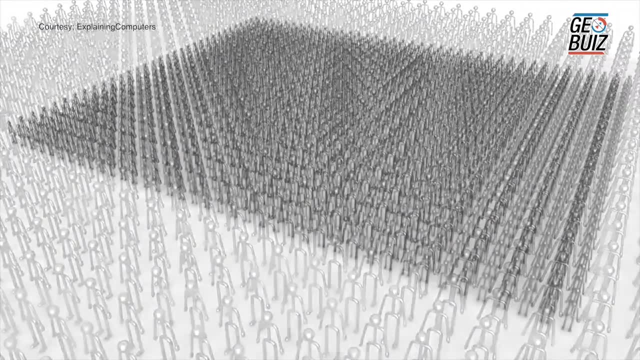 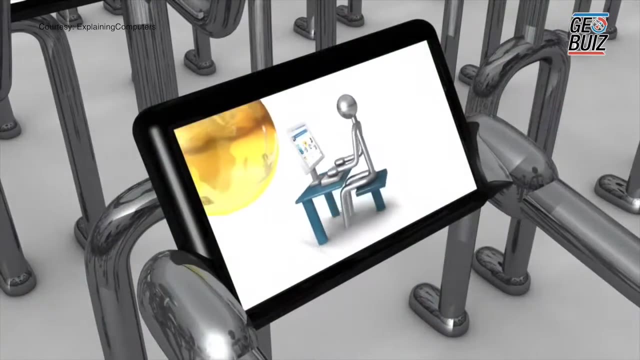 the relevance of big data. now, when we say big data as a technology comes Because big data has an art of dealing with all kinds of data And you can have the architecture where the scalability is all as you grow. So not that you have to plan, let's say for. five years, 10 years. The flexibility is the name of the game. So we have to make sure that as the data grows, we can keep adding capacity to this. So that is where the whole architecture of big data, And then you have two kinds of architecture. So you have the architecture of big data. 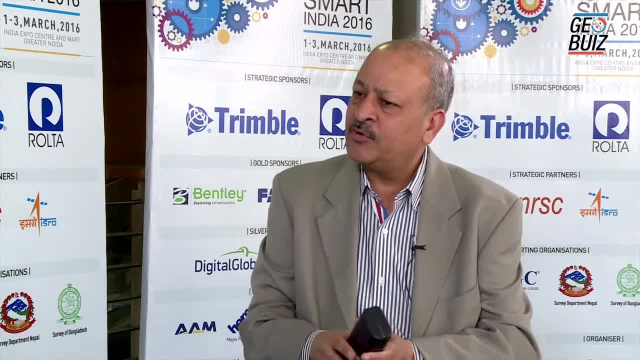 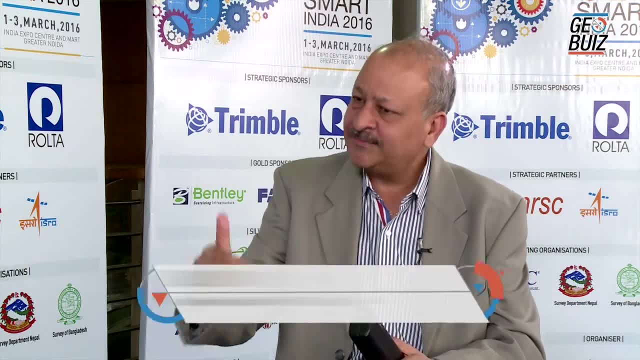 the architecture of big data and the architecture of big data. And then you have two kinds of situations. When you say, big data, you can do it in Open Source, It will absolutely find, But then then there are special devices which helps you manage this technology. and 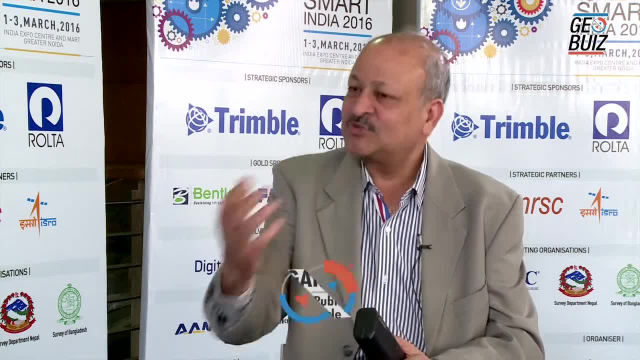 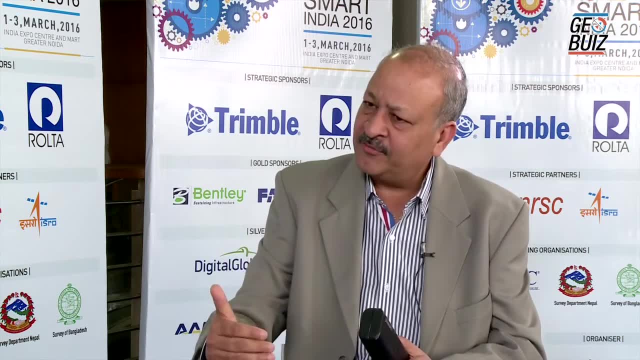 take away the management part or the challenge part and delivers you through the appliances. So that is all about. you know, with technology evolving- And a good thing that happens when you look at some of these appliances that companies in the background keeping in mind- 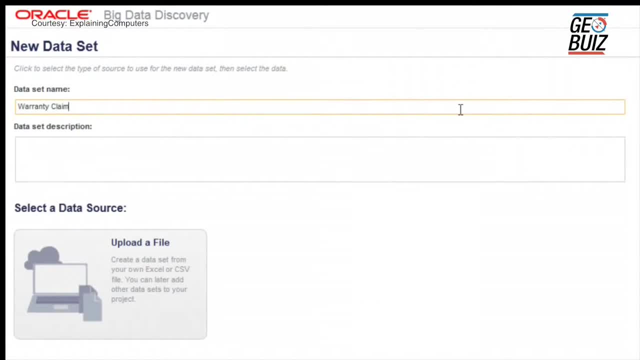 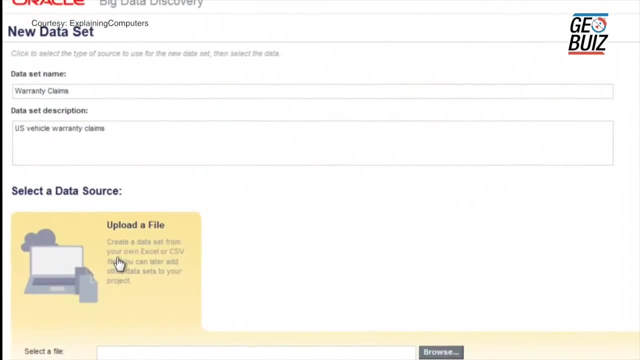 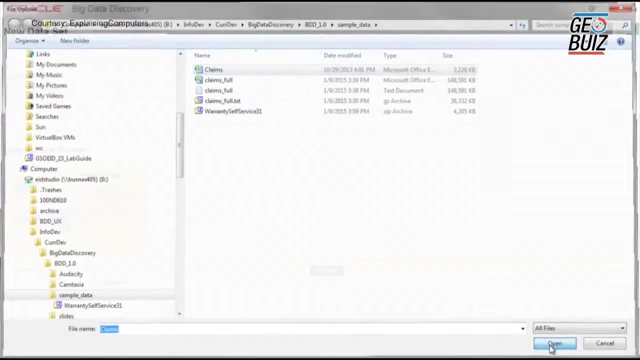 mind the trends. they keep enhancing the capability and capacity of the tech appliances. so you as a user, because your focus is on all about dealing with the data, or you want to deal with the data, you are not interested in dealing with the platform, because that's a separate ball game. 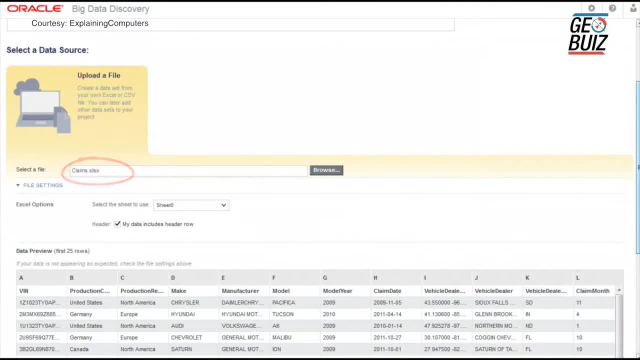 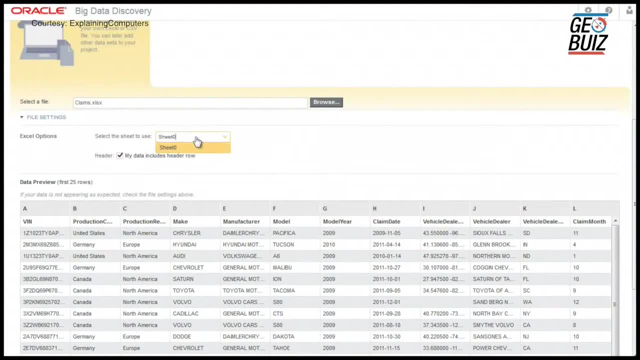 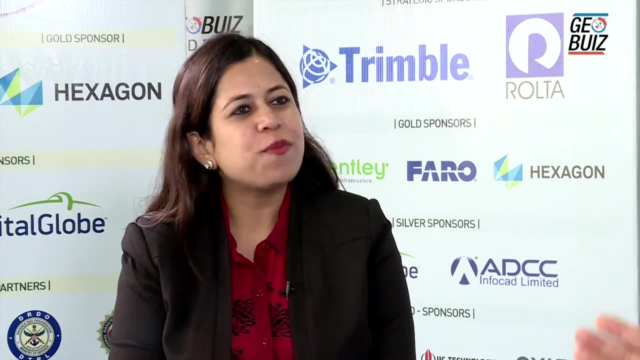 so if you adapt to some of these appliances, the advantages you continue to focus on your business, business needs, business data, the underlying platform, continues to come to you as it innovates or, you know, as it grows. okay, let's talk about our industry now. what is the special? 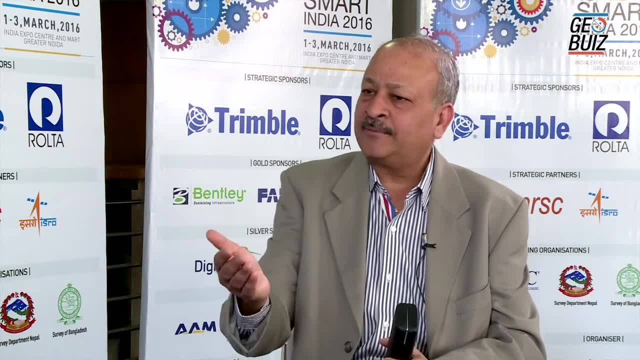 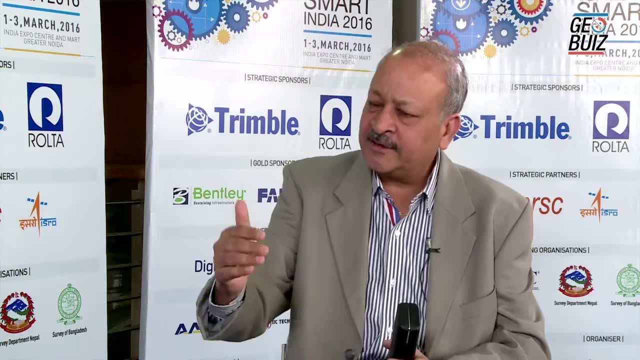 about geospatial big data. so geospatial, if you look at- i will link it back to today- let's say digital india. digital india, if you see right. and let me further take an example of smart cities today we typically see, and i'll just take one example- 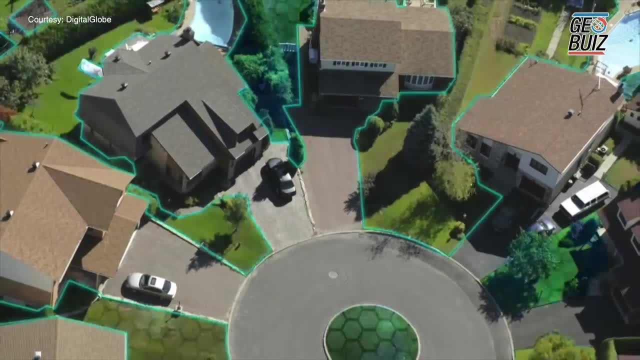 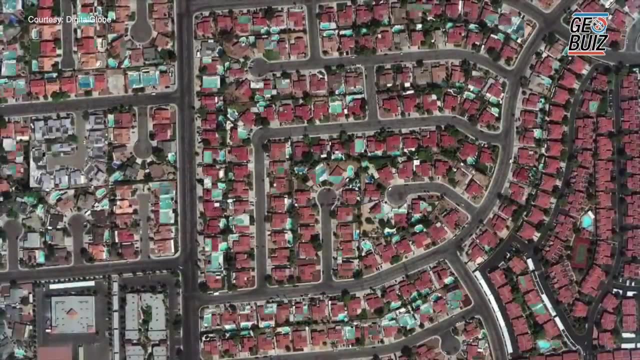 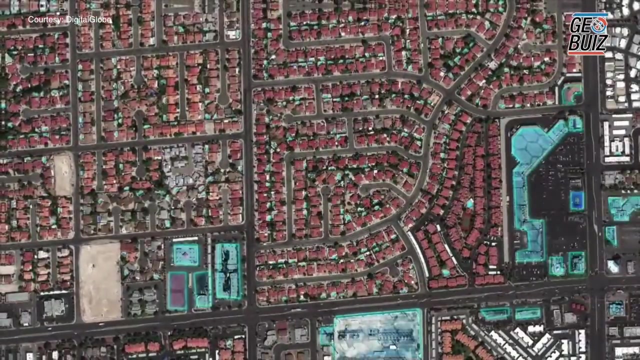 every be month a particular road is digged and then, you know, filled by same department. the next month is, you know, dig by another department and fill in another department, and like that. that is one second. under smart cities we are also doing a lot of planning. so if you do planning in, 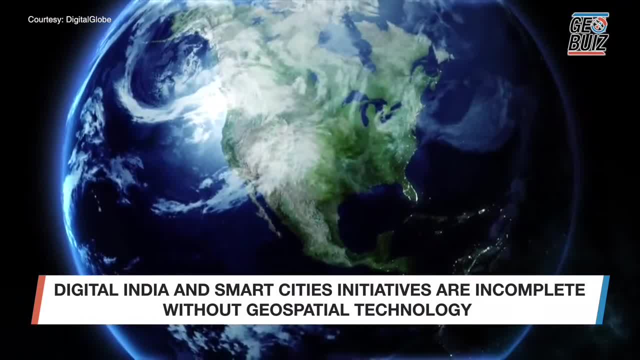 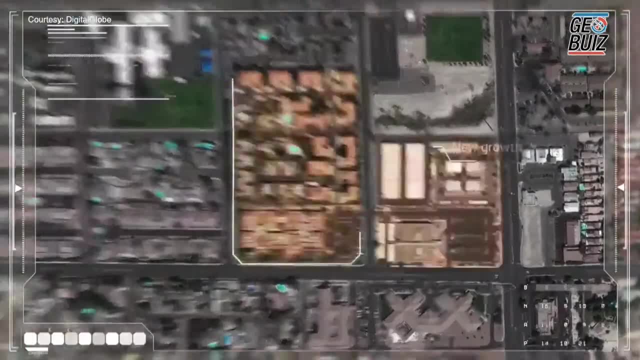 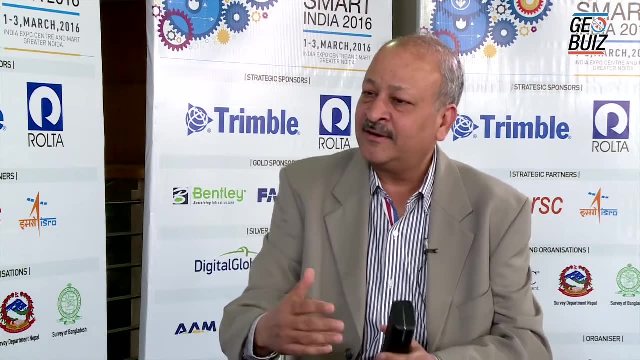 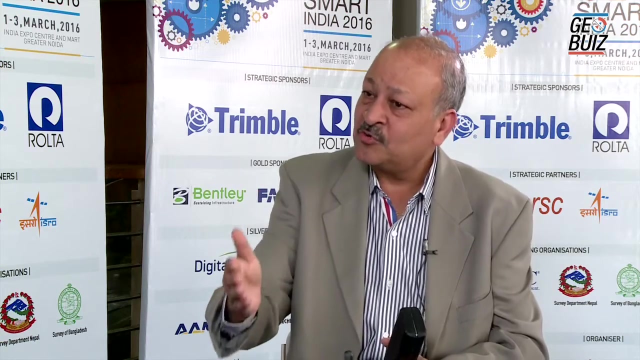 isolation without using, you know, geospatial technology. it is incomplete, so it is necessary to have a policy, not really, rather, some of the smart cities should have a policy actually about you know how should they use geospatial as a part of their plan? for simple reason because if you really want to be smart, you have to do it with the business. 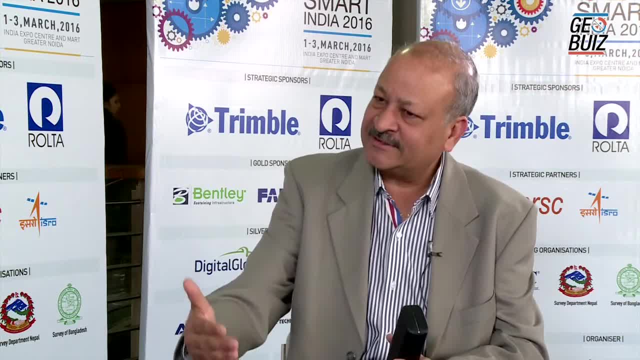 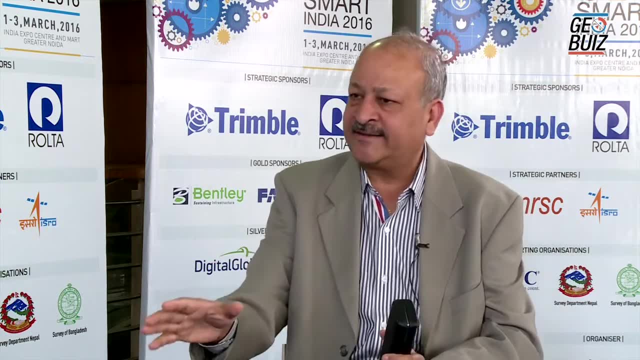 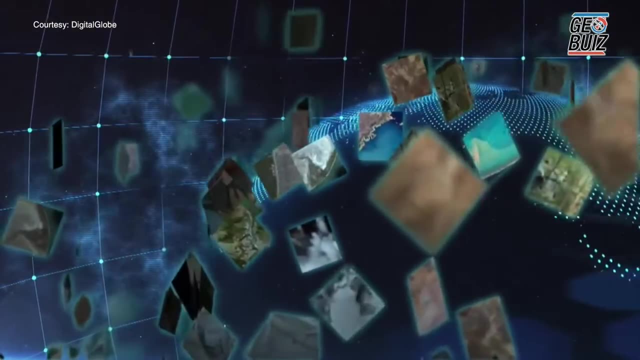 as usual, nuances of today. so maybe through policy interventions they should bring some of these changes into the whole thing. so geospatial has a huge relevance and a huge context, uh, in our industry. because whatever we say, right from planning, through implementation, through maintenance, the whole life cycle, and then you have to keep planning it. because whatever you plan today, every 18 months, two years, three years, five years. you have to review your plans because the requirement keep changing, because what will happen after five years? i'm sure today you can't miss us the way metro happened in country and metro has expanded. i don't think people had. 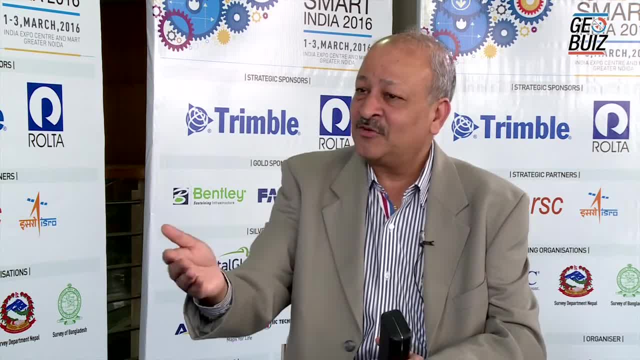 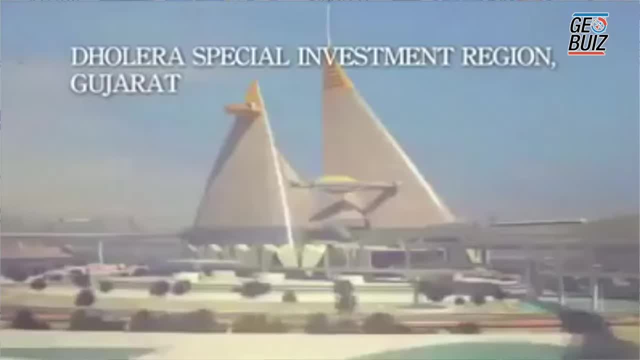 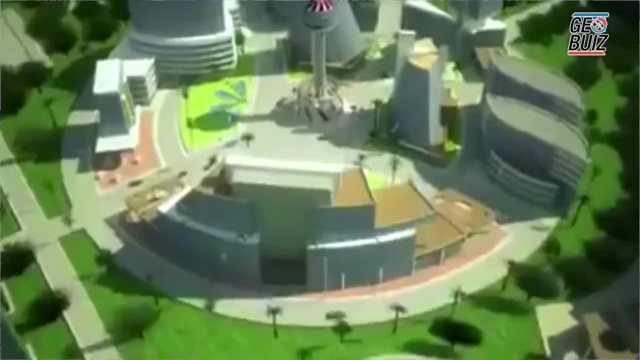 thought at that time. now we are saying, you know, we are saying that we have, the cities are going to grow horizontally. that means they may not be horizontal expansion, but there might be vertical expansion of the city. so either you are going underground or you are going over bridge. so in 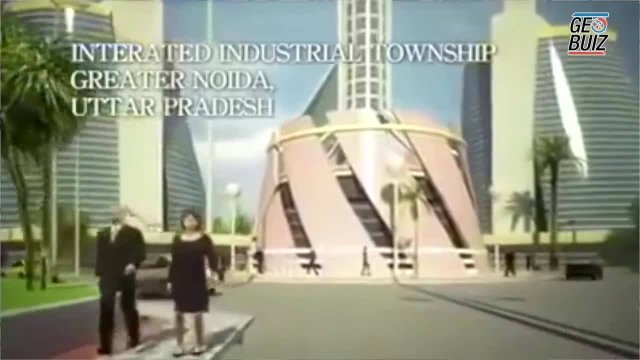 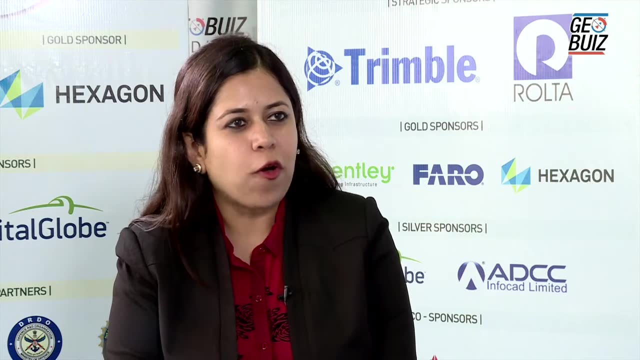 such a scenario. unless you have geospatial in place, you know how will you plan, how will you build this infrastructure. so experts say that you know it's wrong to create bins for geospatial, geospatial big data and the other kind of big data and the process of 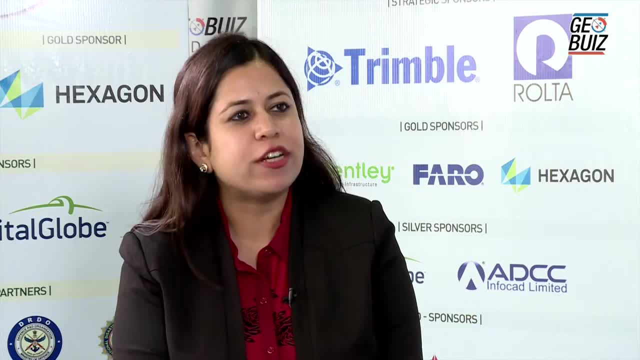 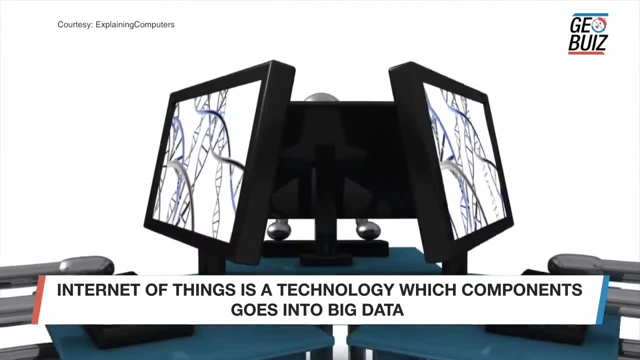 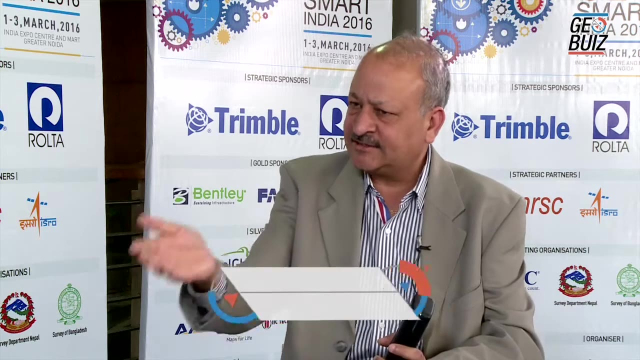 interconnecting various kinds of data through web would ultimately lead to Internet of the Things. What are your views on that? So Internet of Things is one of the technology which the component of that goes into big data. So today, when you say big data, you have audio, you have video, other than structured data, unstructured data, your social data. 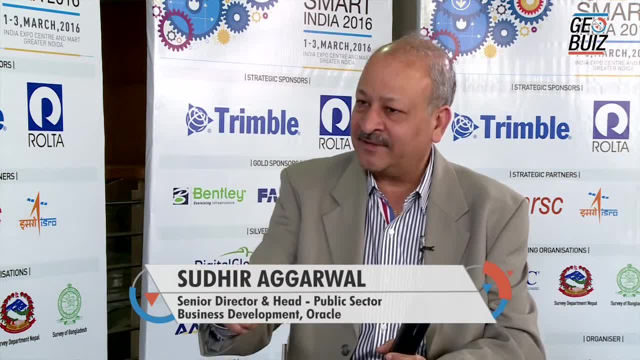 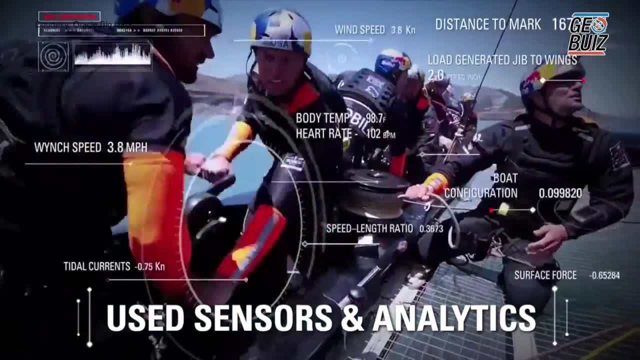 So if you see Internet of Things, and that's where, if you see, with Internet of Things, the velocity comes Because the speed at which sometimes you know you are capturing data through sensors or sensors are transmitting, Now what happens once you get this data? how? 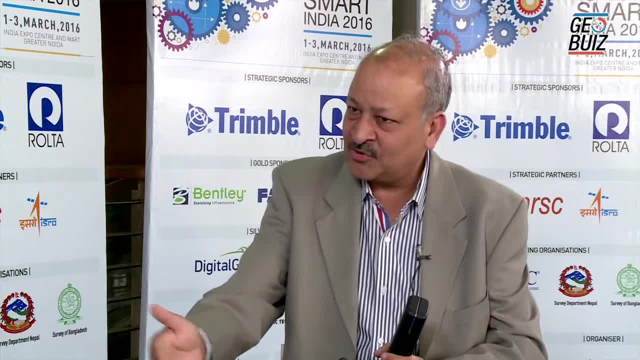 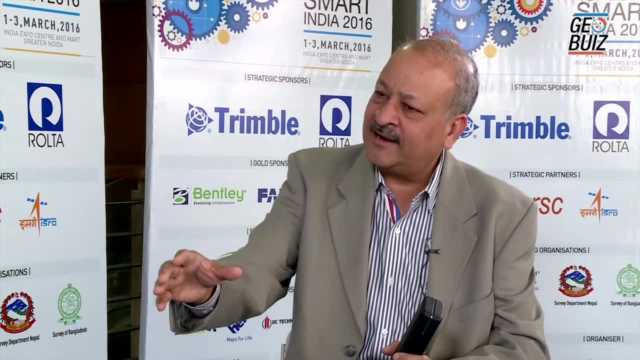 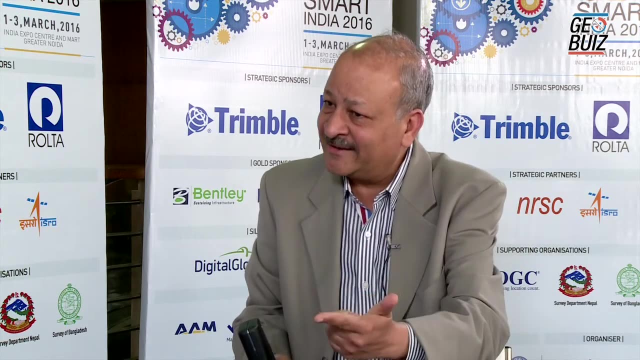 multiple times, in multiple manner this data can be used. So I give an example. let's say, on the river side you put certain sensors. Now maybe you do it from a, let's say, from a clean river perspective. Imagine this data can be used by your agriculture, by your irrigation. 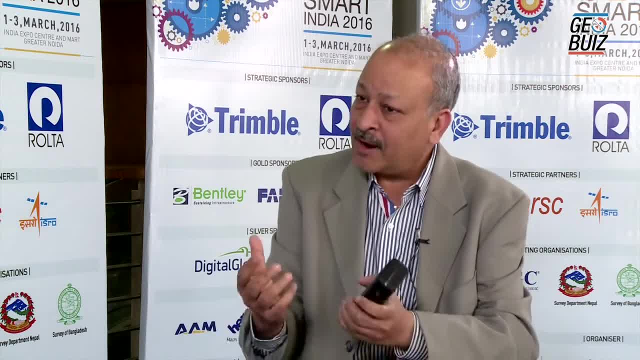 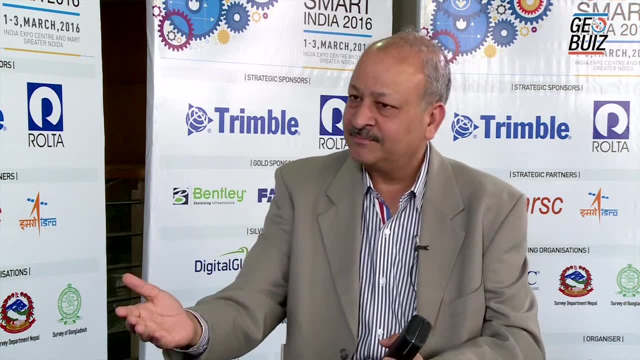 by your climate, by your climate condition, by your disaster management. So the power of the sensor, data and the amount of data it produce at different point of times, So velocity is very, very critical component. and that's where Internet of Things, when we see sensors or cameras- 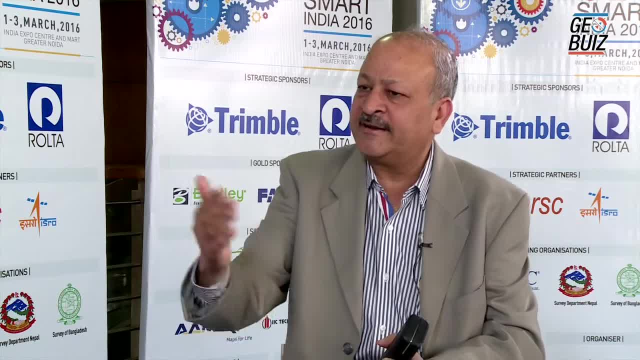 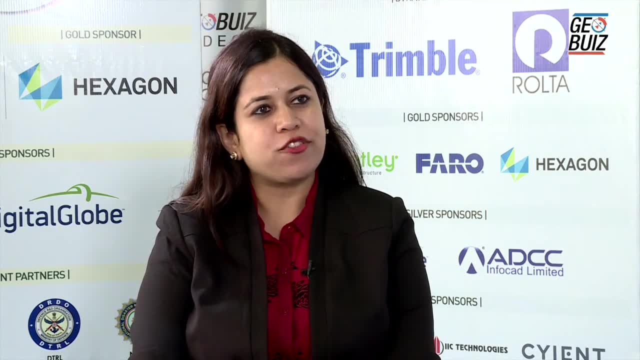 it is going to produce huge data and that's where, like today, you're estimating a data is all your imagination. I can put it back to that. So how can industries take advantage of big data? Industry doesn't have a choice Today. first thing I must say: 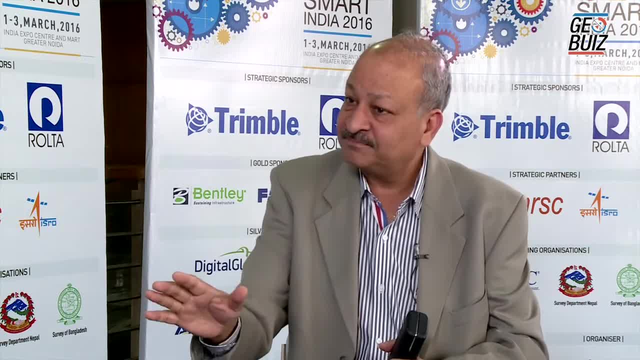 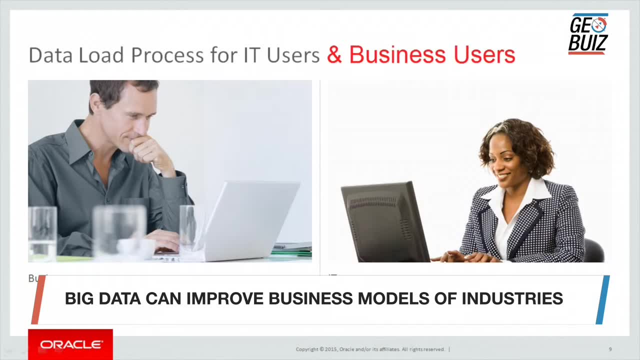 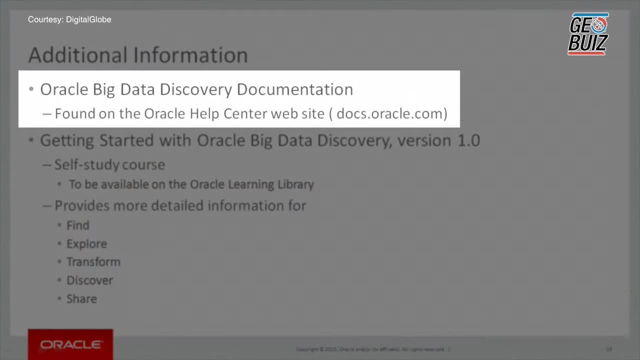 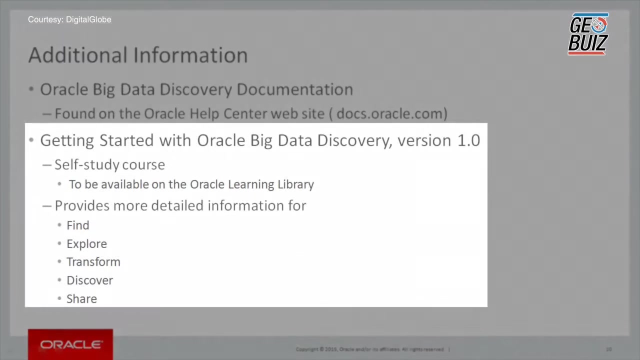 we should not confuse that big data is a technology. To me, big data is a business model, is a strategy, Because days are gone when you used to use this data for your MIS or your analytics. Today, things like big data are dictating and driving your business model. 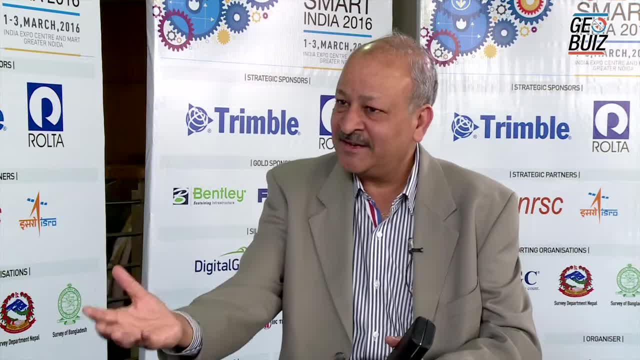 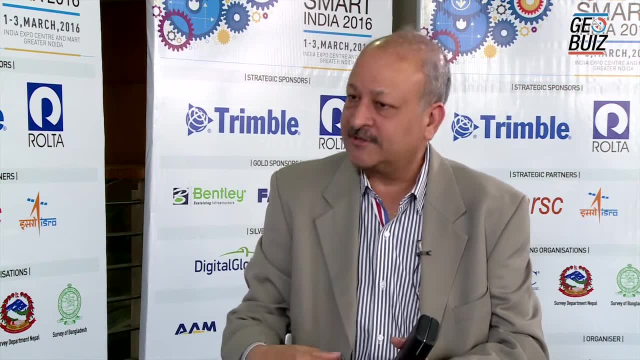 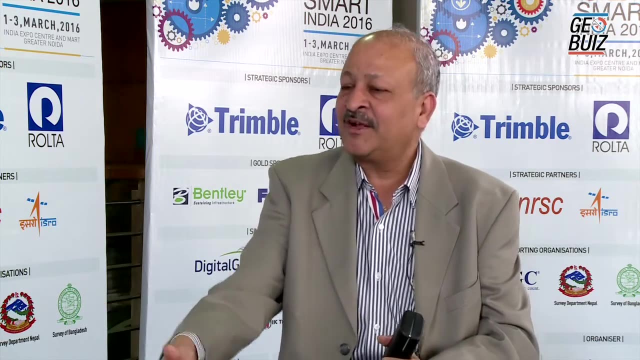 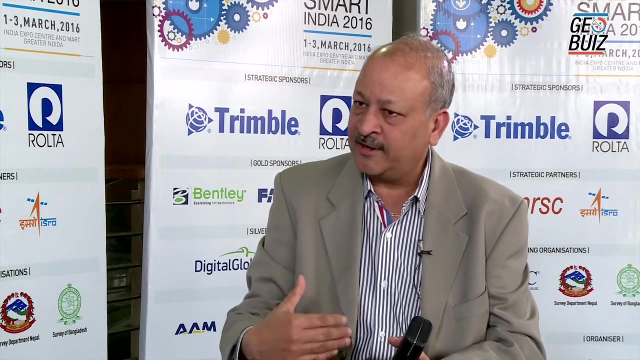 So I call it a digital disruption in a negative context. But if you see positively, digital transformation is leading your business models. Your business models are undergoing change to exploit the power of technology. And that's where I'm saying technology like Internet of Things, big data, should be more viewed as a business tool, business modeling. 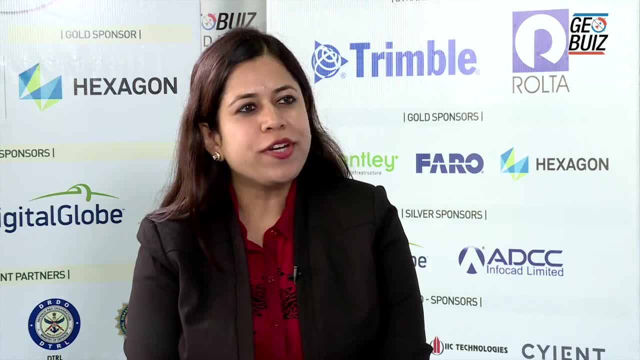 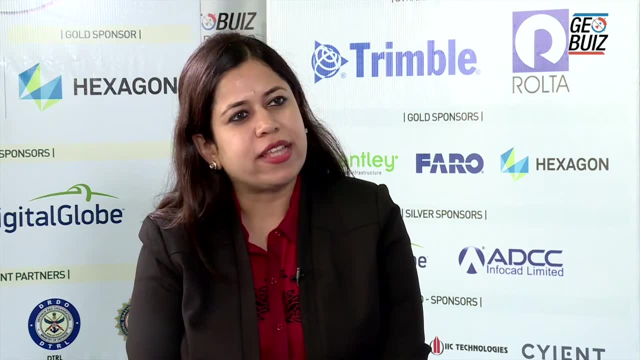 rather than pure technology. So today, you know, if you don't have the tools to analyze it fast, big data can majorly become useless or unmanageable. So how do you deal with something like that? I don't think it's a matter of choice. 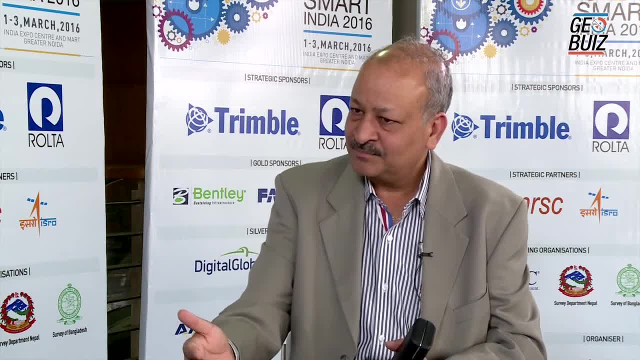 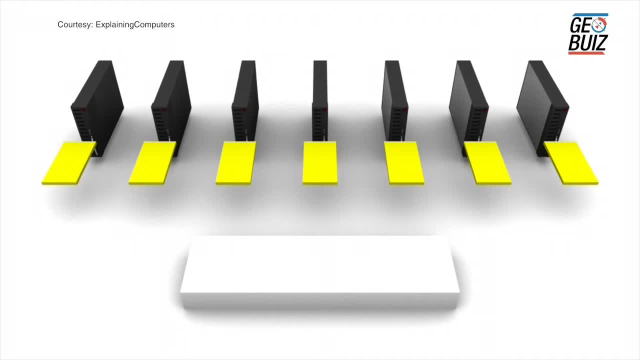 The organization, the people who adopt big data they have, because one is that you know you keep storing data. What do you do with that? So you have to have good analytics And that's where, today, when we say something called smacky, there is a term called smacky in industry, which we say social. 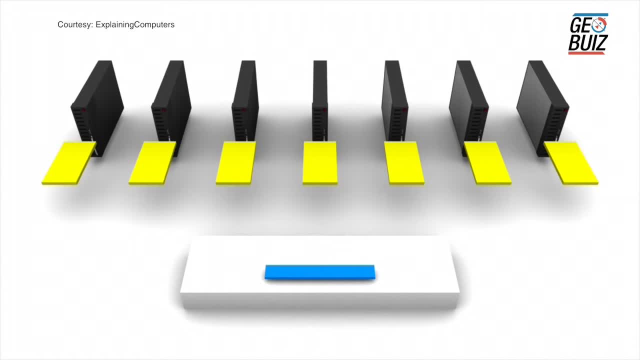 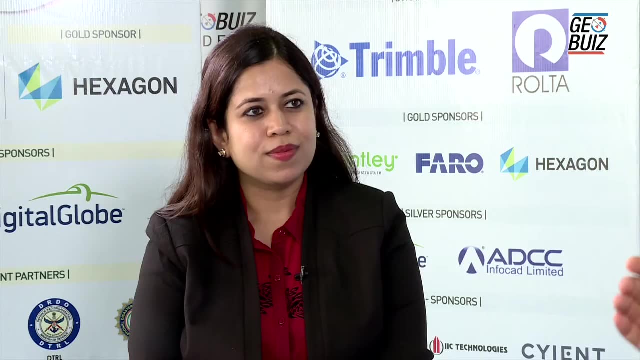 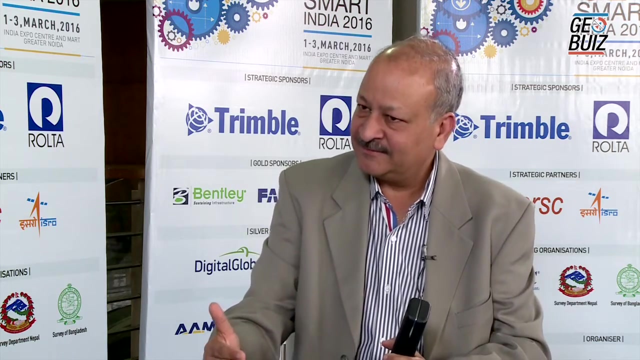 mobility, Analytics, cloud, Internet of Things. So if you see, analytics is actually analytics and big data. If you are adopting big data, you are really impressed by that and you think it's a business need. The corresponding analytics tools have to be in place. 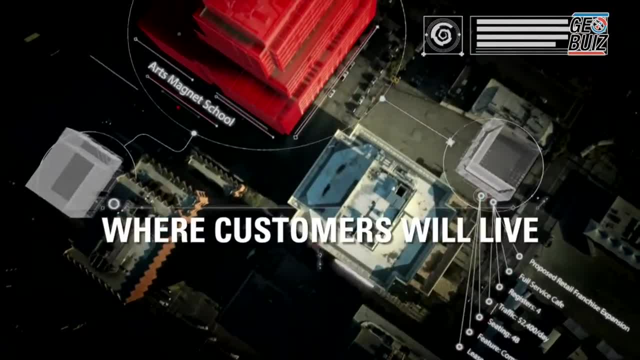 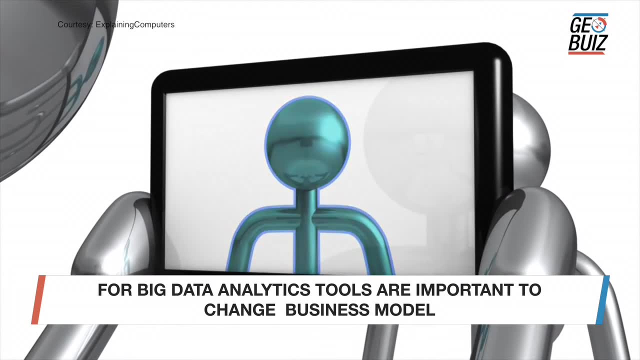 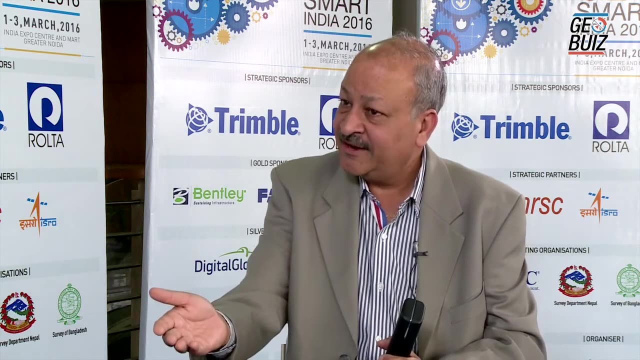 And this analytics is not your typical good old days MIS or even your business analytics. It's a very different kind of analytics which should help you change, maybe change the model of your business, The way you want to do business, what you want to do in business. it may dictate or it may help you.